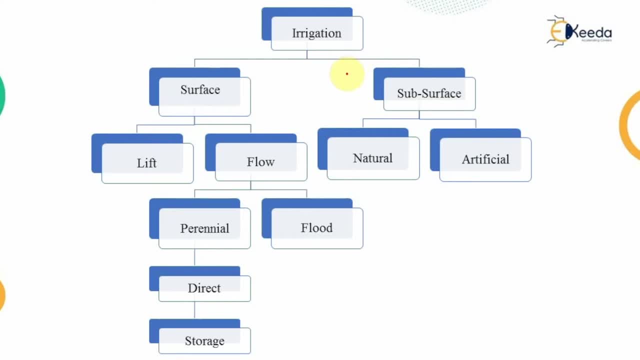 whether it is above the ground surface or below the ground surface. it can be classified into two categories, That is, the surface irrigation and the subsurface irrigation, which is based upon the availability of the water above the ground or below the ground. Then this surface irrigation, the water that can be made to be available onto the ground, above the surface of the earth. 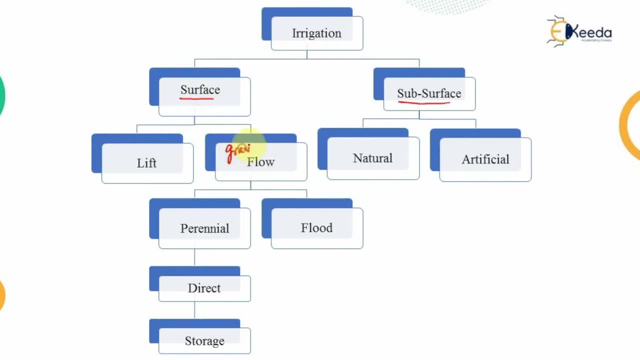 either the method of the gravity that is known as the flow irrigation, or it can be made available using the help of the pumps. Now, if we are using the pumps, that is known as the lift irrigation, because we are increasing the height of the water level. 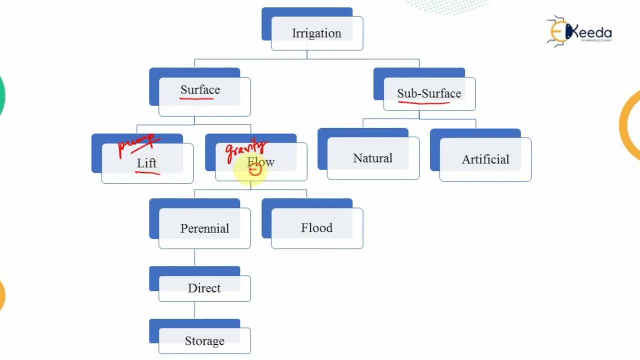 And if it is flowing under the gravitational flow, that is known as the flow irrigation. Now, this flow irrigation, that can be further classified depending upon whether the water is available throughout the year or not. Now, if the entire crop, that field, is flooded with the water, 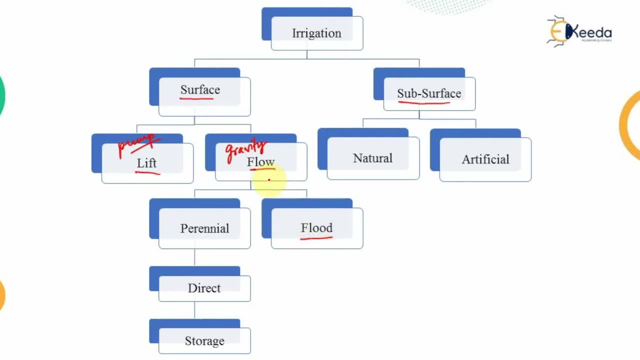 that type of irrigation is known as the flood irrigation. But if we supply only the required amount of water to the crop for the required amount of crop period, that is known as the perennial irrigation. Further, this perennial irrigation, that can be done with the help of the direct irrigation or the storage irrigation. 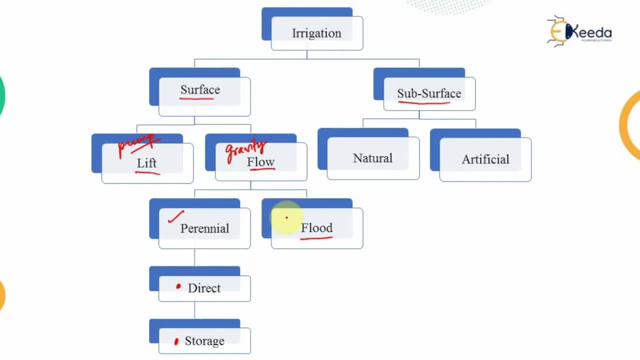 Direct irrigation means if we are supplying the water by directly diverting from the river, while the storage irrigation will be the one where the water is stored into the reservoir before supplying it to the irrigation purposes. Now, one by one, we will look into each of the aspect of the irrigation technique. 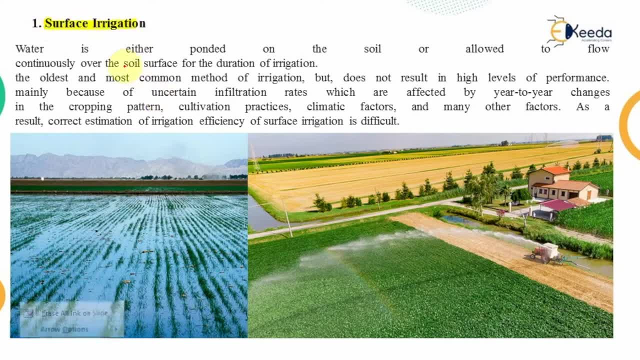 So the first one is the surface irrigation. Now, if the water is ponded on the soil or allowed to flow over the soil, that means what you need to remember here: that surface irrigation means the water will always be present above the ground level. 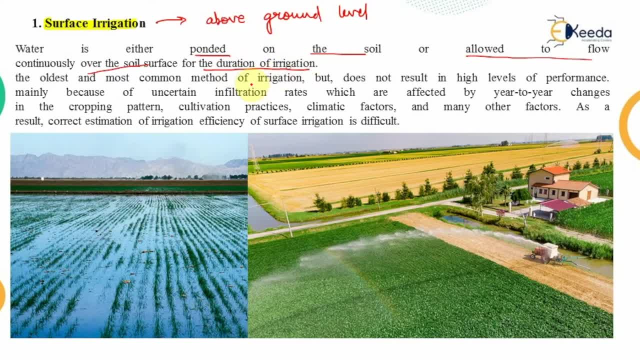 for the duration of the irrigation. The second point in the surface irrigation is that it is the oldest and the most common method, But it does not result in the high levels of the performance. As you can see in the first figure, water is ponded over the field surface. 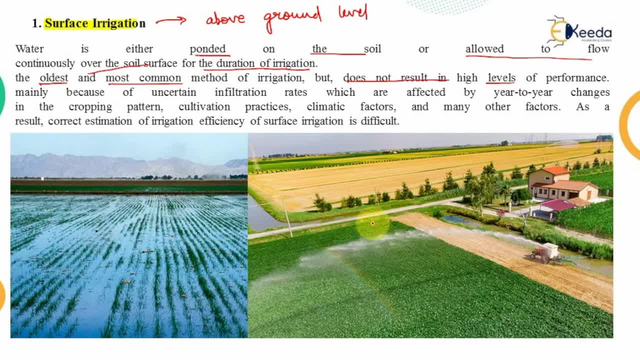 So that is a type of irrigation, While in the second figure you can see that the water is sprayed over the field surface with the help of the pumps. So that is also a type of the surface irrigation, because water is applied onto the surface of the field. 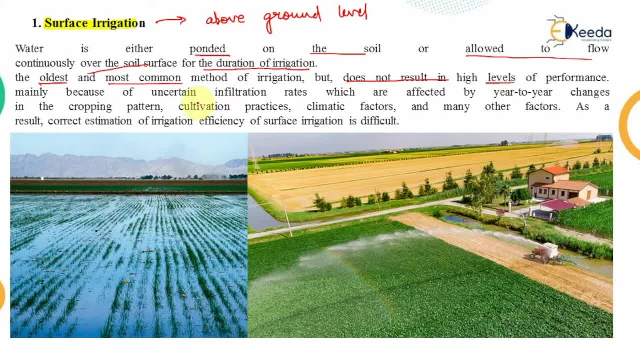 Now why does not it result in the high level of performance? The reason for that is that uncertain infiltration rates, because water has been applied onto the surface but there is certain limitation, as there is certain rate at which the soil in the field will be absorbing the water. 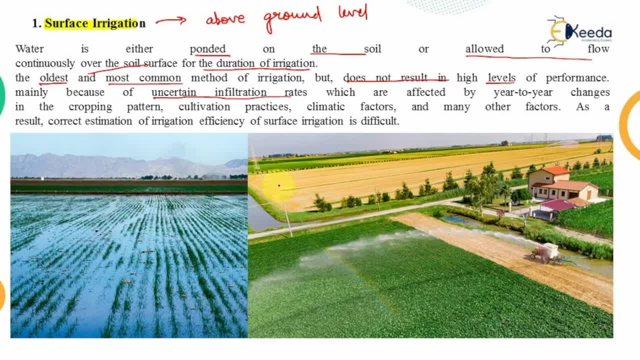 So, depending upon the saturation capacity of the soil- now the infiltration rate is the capacity with which the soil will be absorbing the water and that is affected by year to year changes in the cropping pattern, as well as depending upon the cultivation practices, that which type of cultivation has been done over the field- 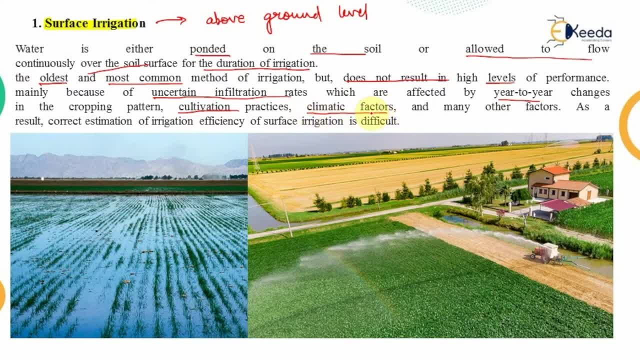 and the climatic factors. If there is rainfall continuously over the field surface, there will be certain infiltration rate, while if there is no rainfall at all, there will be different infiltration rate. So that depends upon the case to case basis. So, as a result, 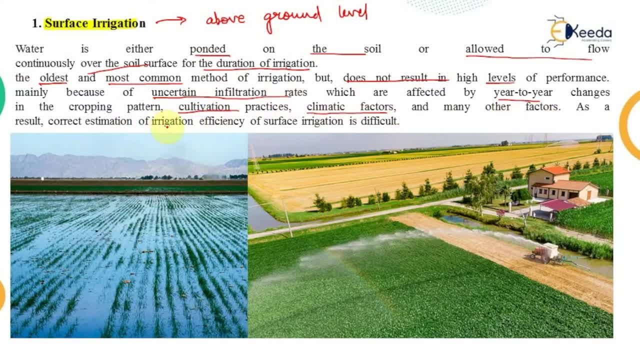 the correct estimation of the irrigation efficiency. that means correct amount of the water that has been absorbed by the soil. we are not able to correctly estimate that, So that is why it does not result in the high levels of the performance. Now this surface irrigation is further classified. 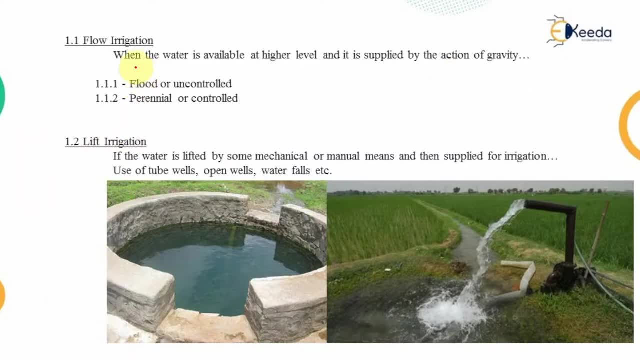 into two categories, That is, the flow irrigation and the lift irrigation. What is the flow irrigation When the water is available at a higher level? That means now, let's say these are the two surfaces at different elevation and the water is ponded over the surface. 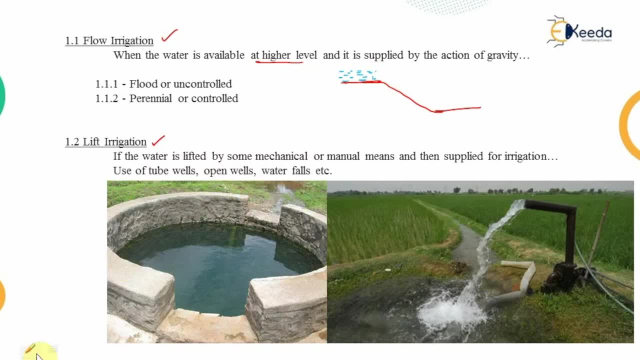 which is higher than the other one And the crop or the field is present at the lower surface. Now, if the water is allowed to fall under the effect of the gravity, such type of irrigation that is known as the flow irrigation, Because water is allowed to flow under the gravity- 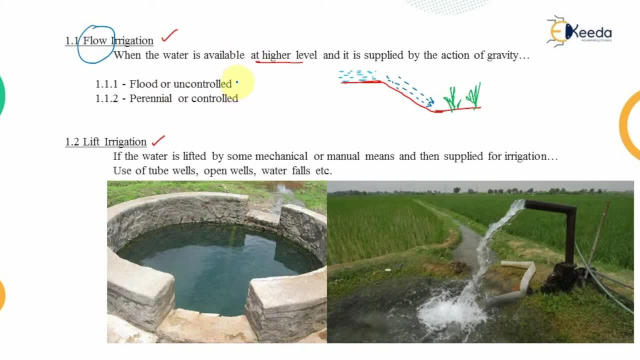 Now this type of flow irrigation is further classified into two, That is, the flood or the uncontrolled irrigation, and the second type is known as the perennial or the controlled irrigation. That we will look after a while. Then, second type of surface irrigation: 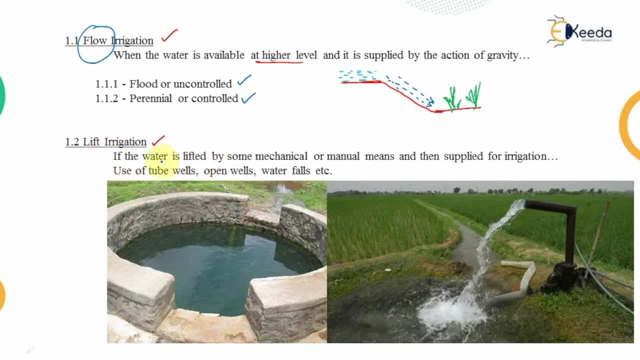 that was the lift irrigation. Now, if the water is lifted by some mechanical or manual means and then it is supplied for the irrigation purposes, Such type of irrigation technique that is known as the lift irrigation, Because we are lifting the water. Now, if the same setup has been reversed, 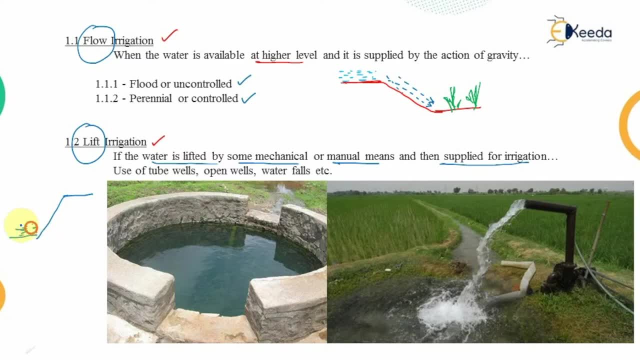 That means the water is available at the surface, which is below, and the field is present on the surface, which is above. Now, in this case, what we need to do, we have to apply the water on to the crops. That means make the water available. 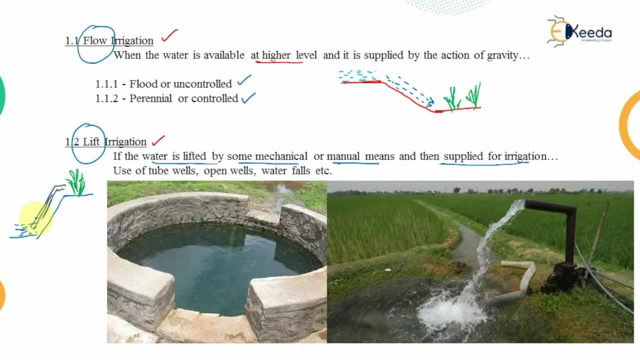 at the higher elevation, And for this we need to take the help of the pumps. And since we are lifting the water to a certain level, that is why this type of irrigation technique is known as the lift irrigation. Now, the common example that you may observe. 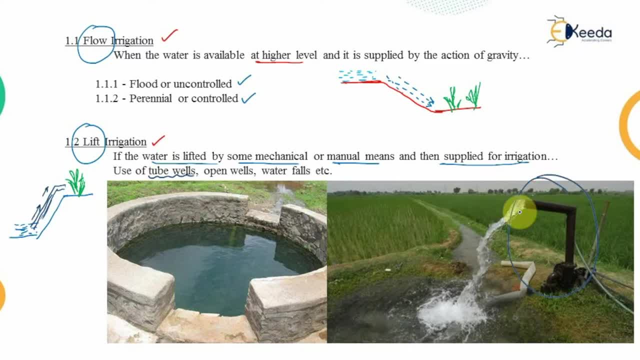 is the use of the tube wells, This type of assembly you might have observed. So the water is present at certain level and that is lifted with the help of these tube wells and then it is supplied for the irrigation purposes. Similarly, the example is the open well. 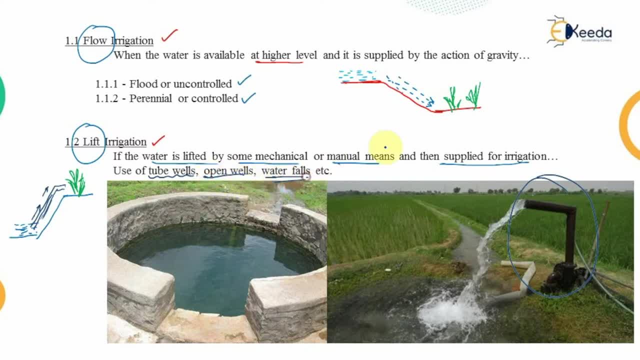 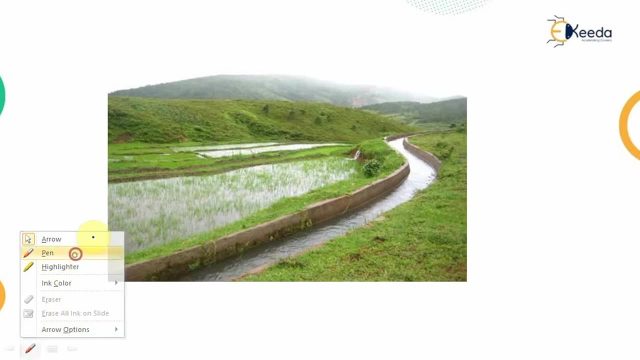 which is available naturally, or the waterfalls, as you might have seen, the water flowing under the different height. that is the example of the lift irrigation. Then this is the example of the flow irrigation. That means the water is allowed to flow under the effect of the gravity. 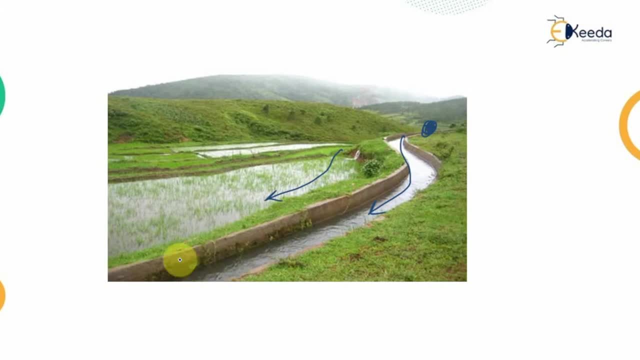 That means there is certain elevation between these two points. Between these two points that I am marking, there is certain elevation. That means this is the change in elevation and because of this change in elevation, which we will not be able to visualize with the help of the naked eyes, 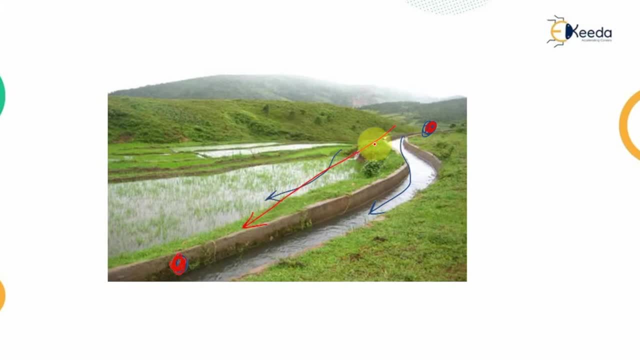 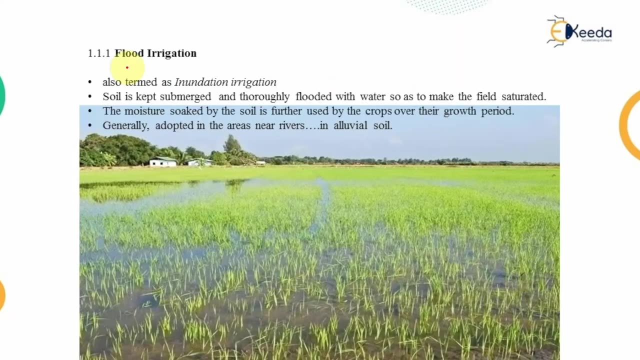 but there will be certain change in the gradient and because of that the water will be flowing under the action of the gravity. Now looking at the different type of flow irrigation. Now, first type of flow irrigation is known as the flood irrigation, As the name itself suggests. 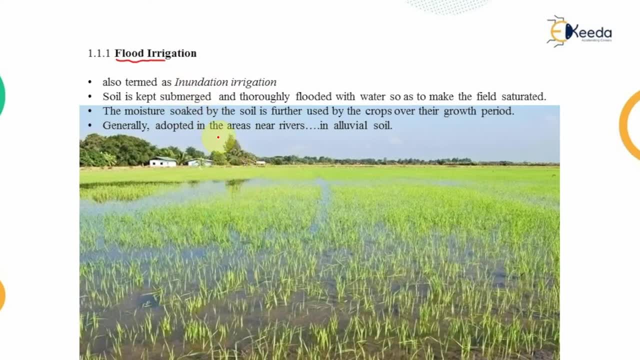 that means the field will be flooded with the water and in this case the soil is kept submerged. that means that is below the water level and thoroughly flooded with the water, so as to make the field saturated. The moisture that will be soaked by the soil is further used by the crops over their growth period. 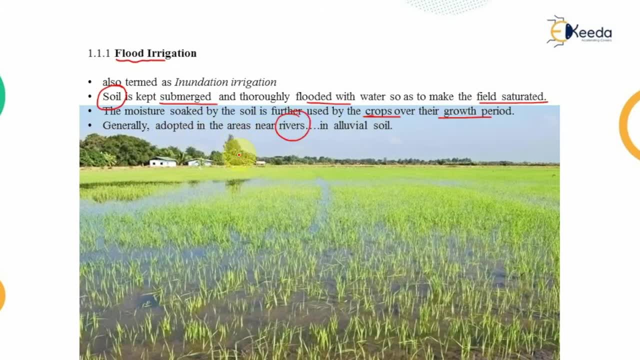 and it is generally adopted in the areas which are near to the rivers, and such type of soil is known as the alluvial soil. And this irrigation technique is also known as the inundation irrigation, where inundation means to flood, The second type of flow irrigation. 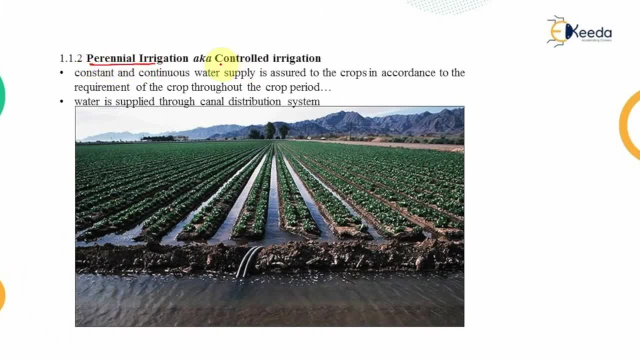 is known as the perennial irrigation, which is also known as the controlled irrigation. That means here the constant and continuous water supply. the water supply that we are having, the amount of that, will be constant throughout the period and it will be for the 24-7. 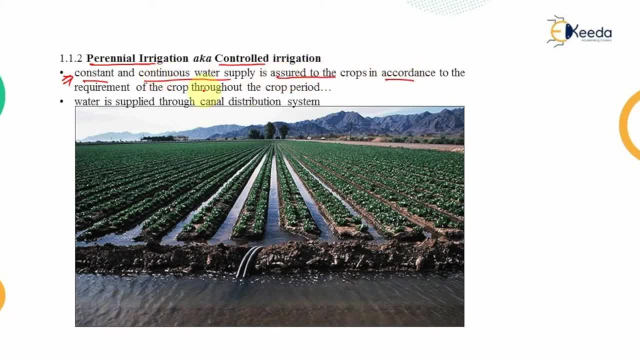 which will be assured to the crops in accordance to their requirement. that means if a crop require 120 cm of the water, then this much amount of water will be available for the crop throughout the crop period. that means for the period for which the crop is present in the field. 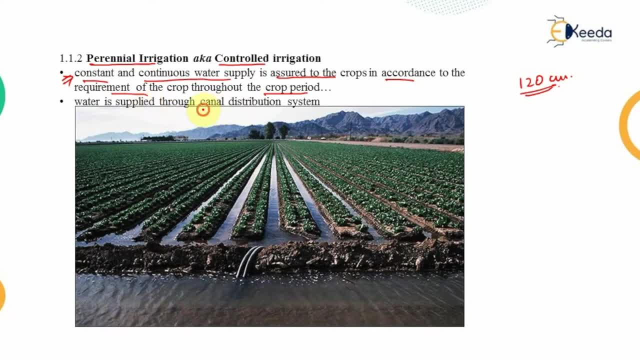 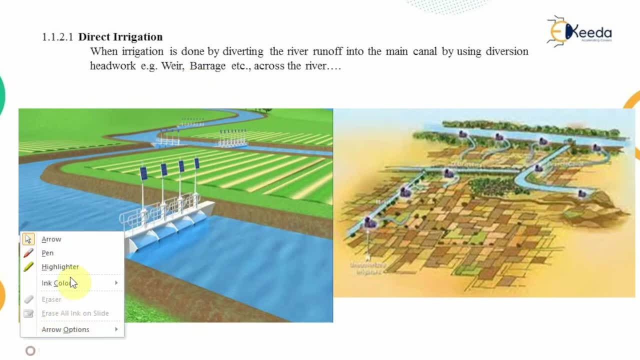 Now, in this system, the water is supplied with the help of the canal distribution system. What is that? So, as you can look at here, the canal distribution system means that there is certain river which is flowing and there is certain canal regulators which are developed. 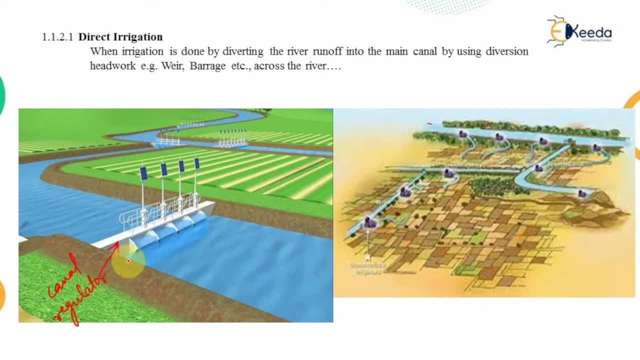 This we will see in the later stages of the course. So these canal regulators are built over the river. Now what they do? They stop the flow of the river and this stopped water that is diverted into the another tributaries or another canals. 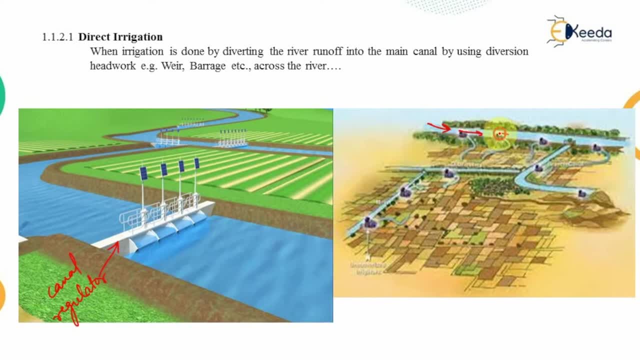 Now, as you can see in this image, the water is flowing through this river and this water is diverted into certain other canals. Now these canals are flowing through the fields. then another canal is taken from that main canal, which is known as the branch canal. 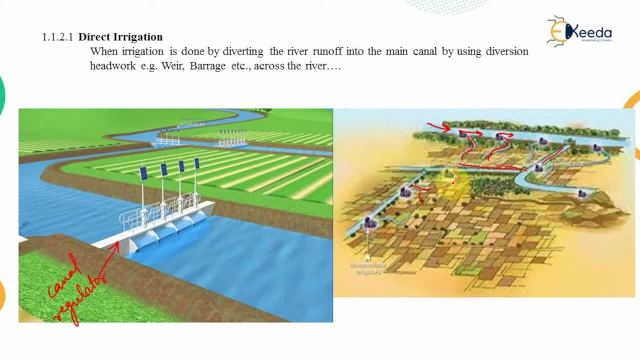 Then further branch canal is distributed into the different number of miners or the distributors. So such is the type of the system, and this entire system is known as the canal distribution system. Now this perennial irrigation that is further classified into two. That is the direct irrigation. 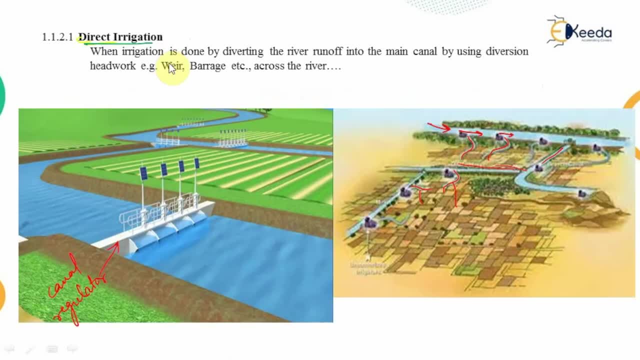 and the second one is the storage irrigation. Now, if you look at the direct irrigation, when irrigation is done by diverting the river runoff into the main canal, as I have shown in this image, that means this was the main river and that flow was diverted into the canal. 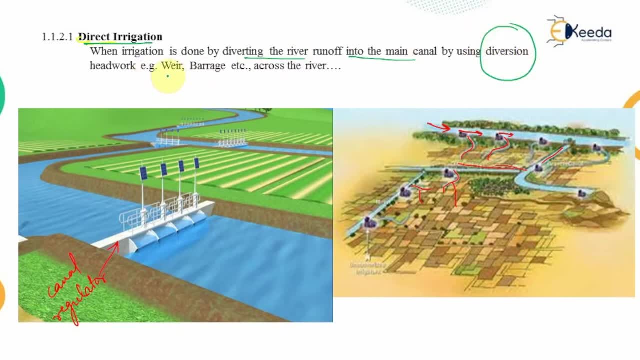 by using the diversion headwork. Now these diversion headwork are known as the weir or barrages, and they are built across the river, So such type of irrigation system is known as the direct irrigation, While in this storage irrigation we construct a dam. 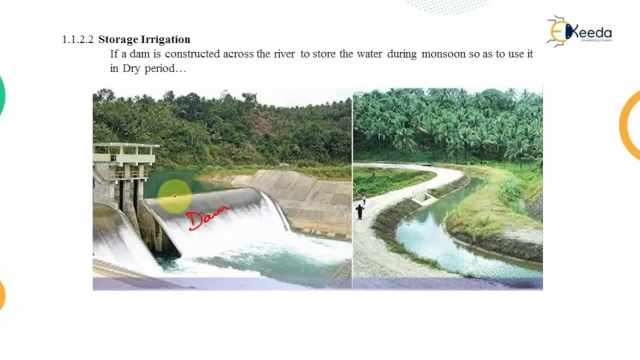 This is a dam which is constructed Now the water that will be stored behind the dam and that store, or the pool of the water that is known as the reservoir. Now, that reservoir will be storing the water during the monsoon, The period in which there will be flow of the water. 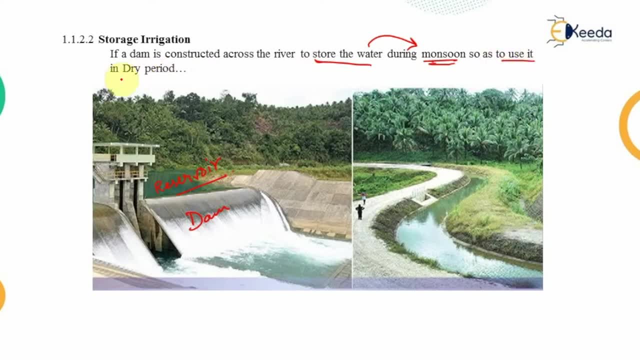 Now that stored water is used in the dry period. So if we are storing the water, that is the storage irrigation, but if we are directly supplying it into the field, that is the direct irrigation. So that completes the first type of irrigation technique that is known as the surface irrigation. 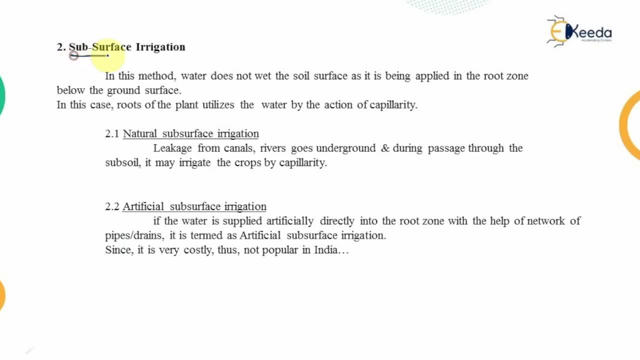 The second type of irrigation technique is known as the subsurface irrigation. Now, in the name it already suggests that the water that will be applied if this is the ground level and this is the crop Now, this is the root zone of the crop and this is the crop which is growing over the field. 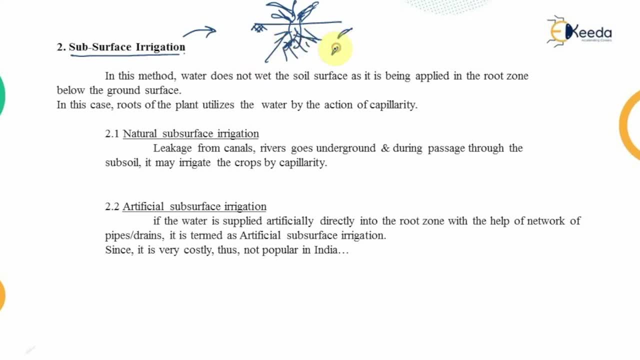 So this is the root zone, So the water will be applied into the root zone. So in this case the water does not wet the soil surface. That means the water is not applied on the soil surface, It is applied in the root zone below the ground surface. 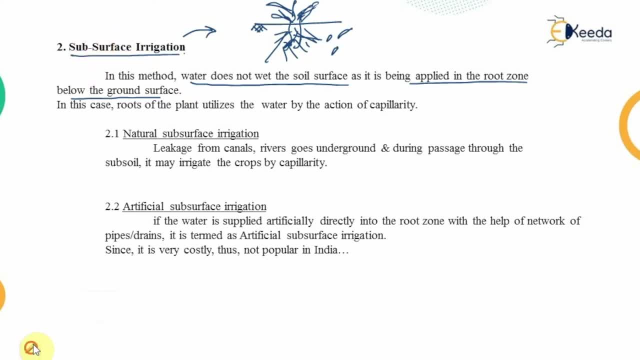 The water is applied below the surface. that is why the name comes as the subsurface, Now the roots, which are present below the surface level. they utilize the water by the action of the capillarity. Now, this capillarity is the phenomena with the help of which 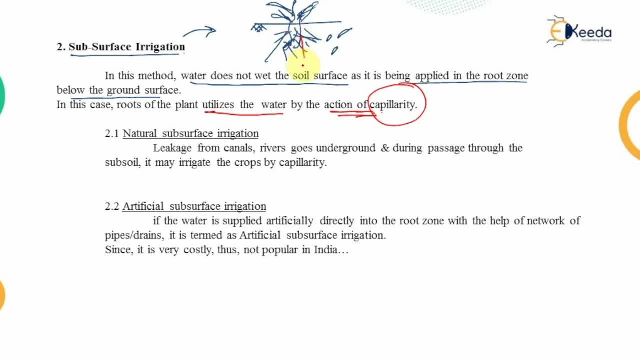 they suck out this water and use it for the photosynthetic purposes. Now, first type of subsurface irrigation. that can be either through the natural means or through the artificial means. Now, what is the natural subsurface irrigation? Now, if you look at the cross section of the canal, 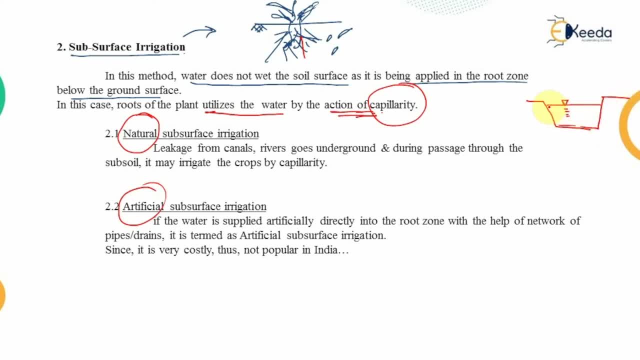 This is the canal. Now, in the natural subsurface irrigation, there are the probability of the leakage from the canals or the rivers. Now this leaked water from the canals or the river that goes underground and when it is passing through the water table, or that means the area that is known as the subsoil area, 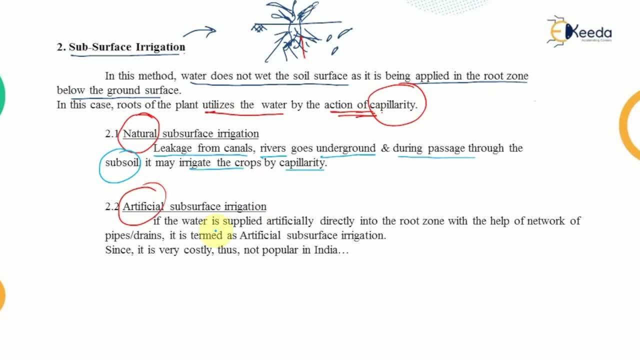 then it irrigates the crop by the capillarity action. Similar action is performed in the artificial subsurface irrigation. The only difference is that now, in this case, we are deliberately supplying the water directly into the root zone. Now, for this, we need to establish a certain network of the pipes or the drains. 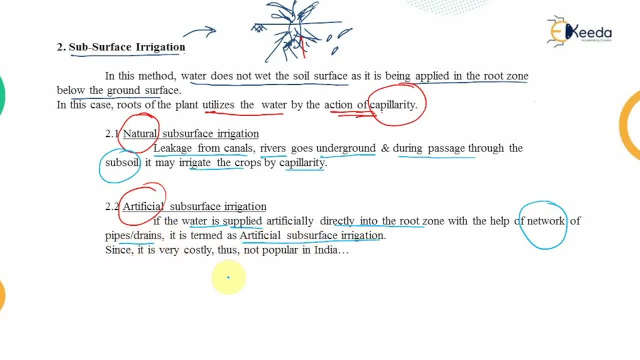 and this type of system is known as the artificial subsurface irrigation. Now, if we are directly supplying the water into the root zone, that means we need to establish this network, and this network of the pipes or drains is established below the ground surface. That's why it is very costly. 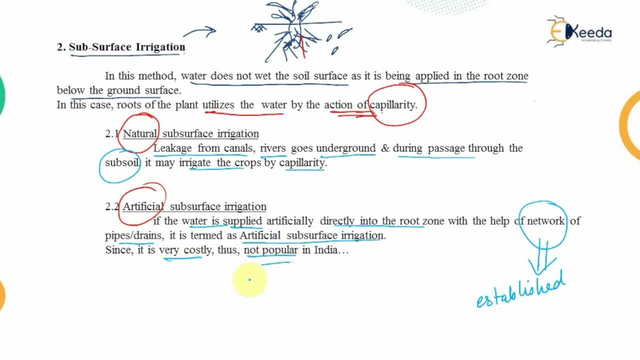 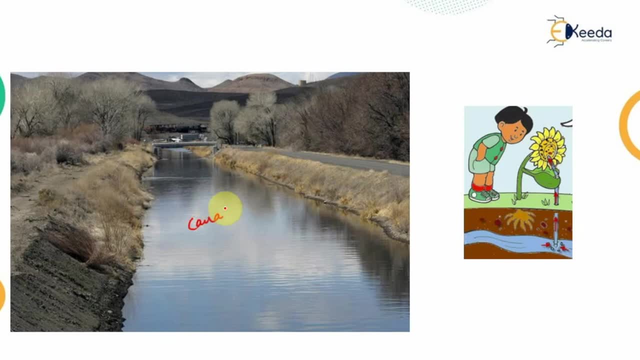 and that is the reason that it is not very popular in case of India. Now, if we look at these images, this is the canal or the river. there is a certain earthen boundary which is constructed over here. Now, if you look at the cross section over here,